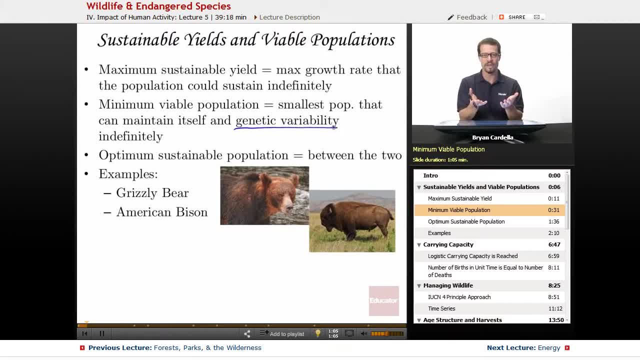 variability indefinitely When you have just two left and their responsibility is to regenerate a more abundant population of that species. that's a lot of pressure in terms of genetic variability Because in a sense, it's inbreeding when there's just two left. So you're not going. 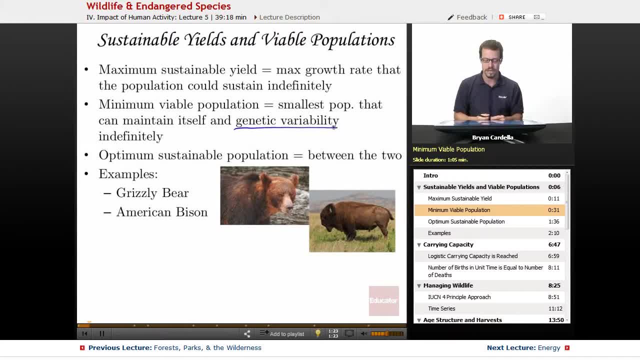 to get that genetic variability that's desirable in the long term for a population. They'll be extremely vulnerable to it. So the maximum sustainable yield and minimum viable population is going to vary depending on the organism we're talking about. In between those two is the optimum sustainable population, So it's. 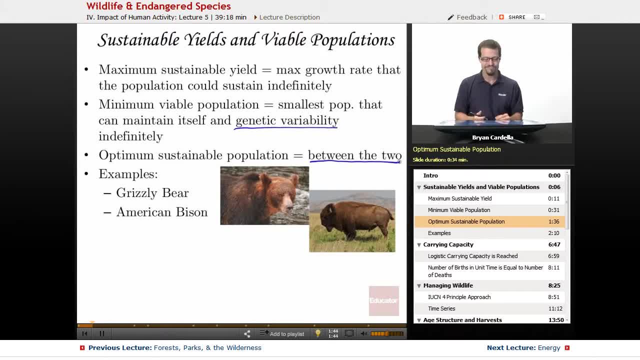 between the two. It's that, in a sense, happy medium. It's not reasonable, especially if a species is threatened or endangered, to get up to the maximum sustainable yield. That may not be feasible because the area that it used to live in is not the area that it used to live in, And so 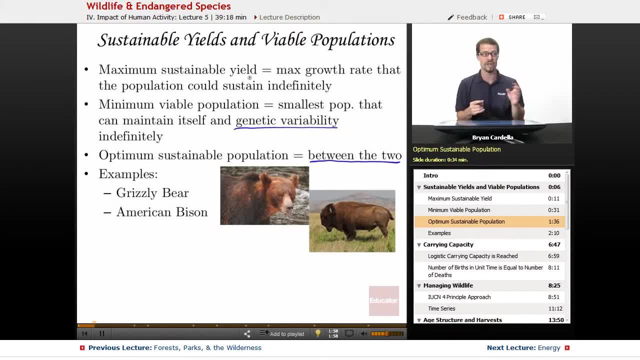 it's not the area that it used to exist in. A lot of it is now human civilization, or a lot of that forest has been destroyed. But on the one hand, we don't want to get down to the minimum. So having some kind of optimum in the middle is what a lot of scientists or environmentalists are shooting for. 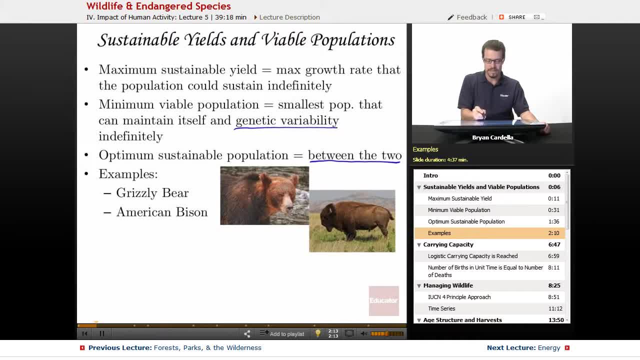 Here's some examples with the grizzly bear and the American bison. The grizzly bear is fascinating to me. I live in California. It's on the state flag, But there are no grizzly bears in California anymore. There used to be a lot of them in the United States. 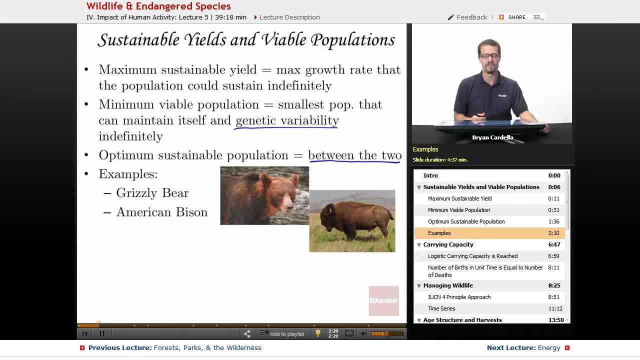 The grizzly bear is fascinating to me. I live in California. It's on the state flag, But there are no grizzly bears in California anymore. There used to be a lot of them in the United States. Not so much anymore. You have to go up into Canada to see a grizzly bear, So they're definitely endangered. 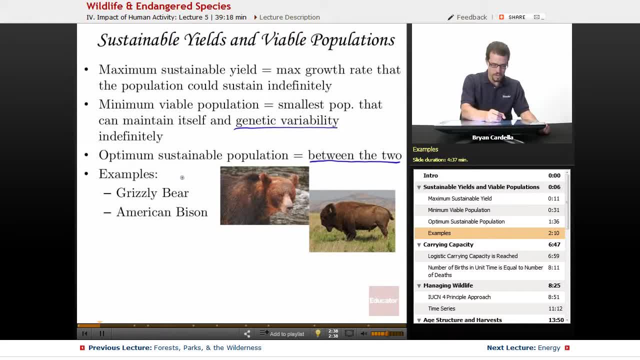 And some little facts. When you're looking at the females, you're seeing All men are about 300 pounds, With males up to about 600 pounds. Full grown ones with hind legs are 8 ft tall, but bears are 800 pounds. if all three areoh, that's pretty intimidating. And full-grown bears are 8 ft tall. if all three areoh, that's pretty intimidating. And full-grown bears are 8 ft tall if all three areoh, that's pretty intimidating. part of the reason they've been known as grizzly bears is class summers. 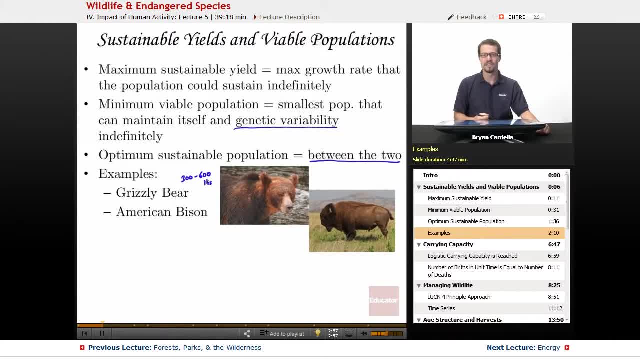 part of the reason they've been known as grizzly bears is class summers. Part of the reason they are endangered is, well, they were considered a threat And a lot of them were hunted for and killed, more so than probably should have. 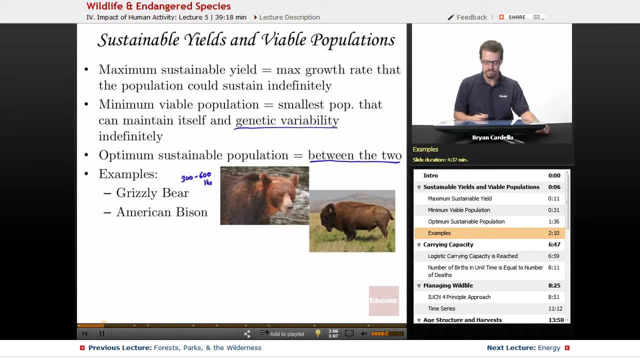 And that's why we don't see them as much in the United States. So how can we estimate where the grizzly population was If we go back to the 1800s? we don't have a time machine, obviously, But in terms of records that were kept, 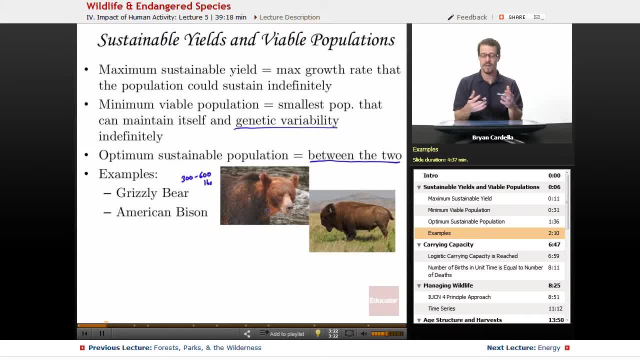 we don't have exact numbers And they wouldn't have been able to give us exact numbers back then. but we can look at Lewis and Clark's expedition, So in the 19th century, in the early 1800s, when they made that expedition to the West Coast. 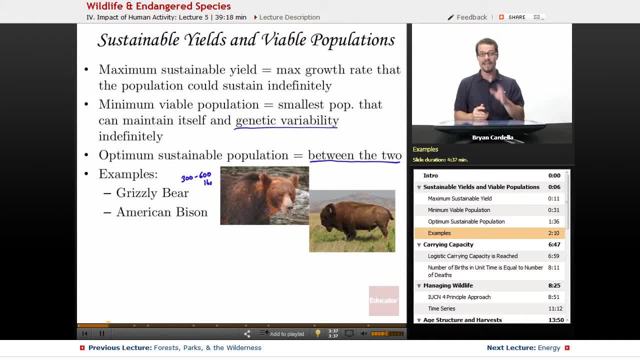 they kept track of how many grizzly bears they saw, And they were actually very specific. When they passed buffalo or bison, they would just say, oh, there's a lot of them over there, Because they weren't as much of a threat. 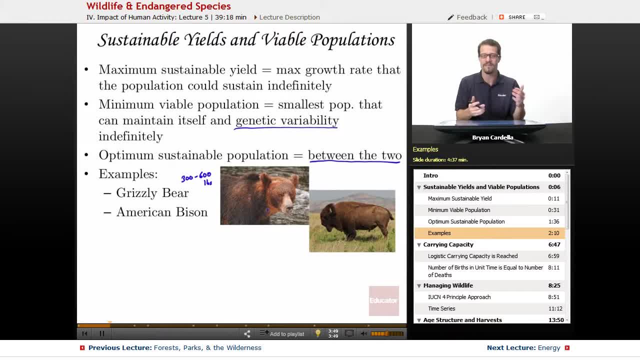 They didn't care to figure out. hey, are there 1,000 bison? Are there 5,000?? They just would say there's a lot of them, But with grizzly bears being surprised by seeing one and the potential threat. 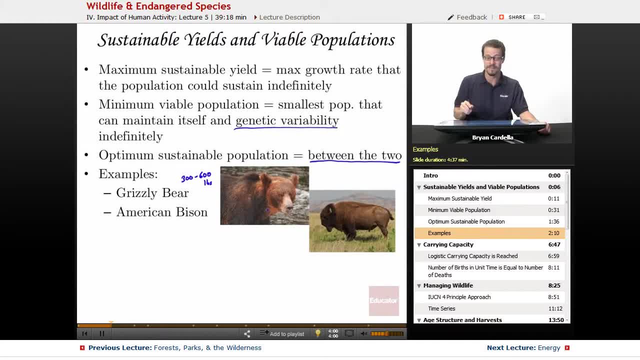 they made note in their journal. we saw a grizzly bear today, We saw three of them today And when you add up the total number in their journey they encountered 37- over 1,000 miles that they traveled. They kept miles in their journal rather than kilometers. And so that comes down to about 3.7 grizzly bears per 100 square miles, And if you consider the space where grizzly bears existed back then, they've come up with a calculation that in the early 1800s there were about 12,000 grizzly bears. 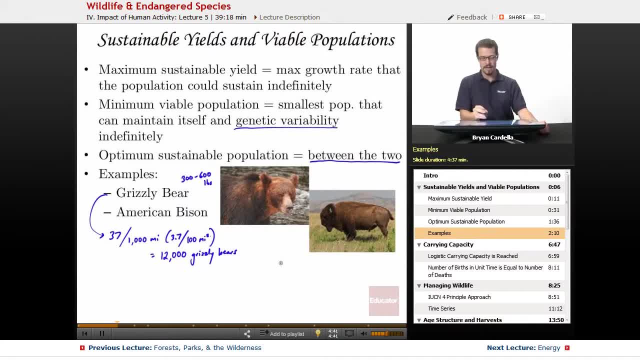 There are significantly less now, But they are protected And hopefully, because of human intervention and regulation in terms of preserving them, we can get back to a reasonable number: 12,000 grizzly bears. It may not be reasonable at this point in time. 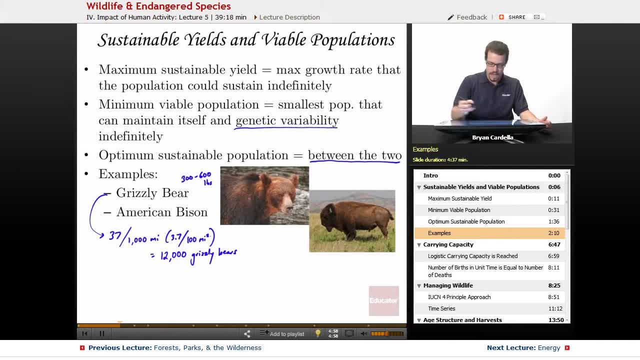 When we look at the American bison- slightly different tale- We've been able to bring back the American bison to fairly high levels in terms of their overall population numbers. We're certainly not at the maximum sustainable yield. We're not going to go there again. 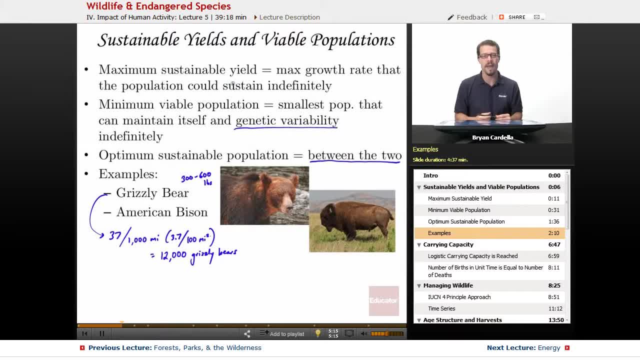 Because in the mid-1800s we're talking millions, millions of bison roaming the plains. A lot of Native American Tribes depended on them directly And during especially the middle of the 1800s into the 1870s, a lot of bison were hunted by white Americans.